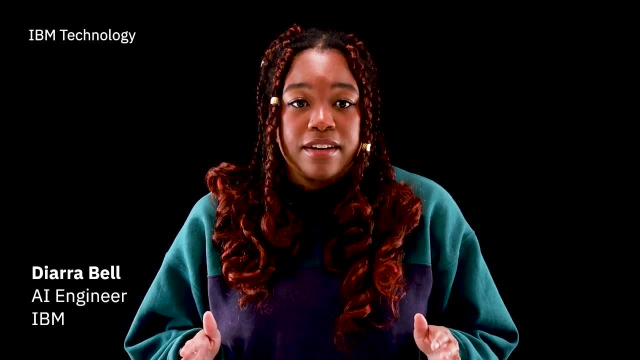 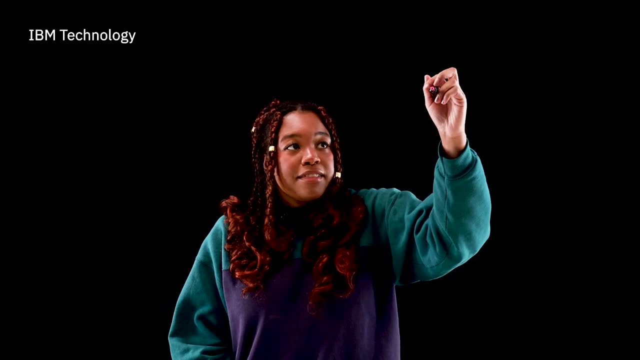 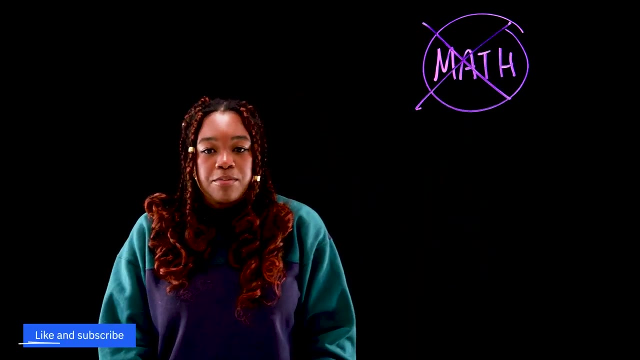 I have a confession to make: I don't like math. Well, at least if you're like me, you might not like pure theoretical math. Whenever I would be sitting in my math classes like calculus or algebra or trigonometry- I always wondered if I would ever have to use these concepts. 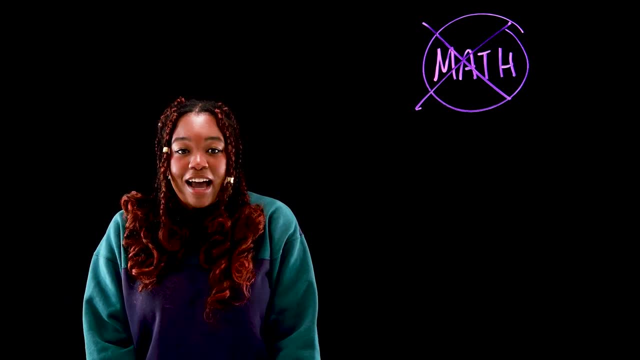 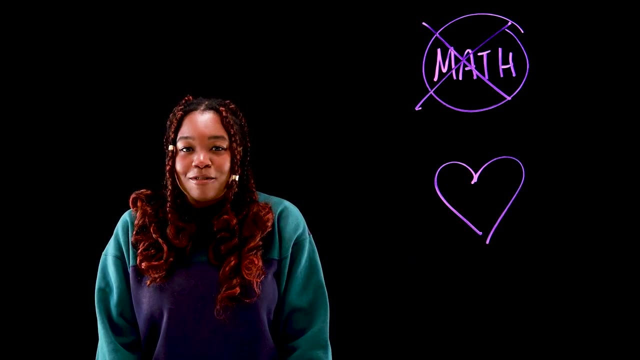 However, if you're like me, you might love computer science. I love computer science because it helps us explain math topics in a way that's easy for our computer to understand, and that makes it a little easier for me to understand too. That's important because when 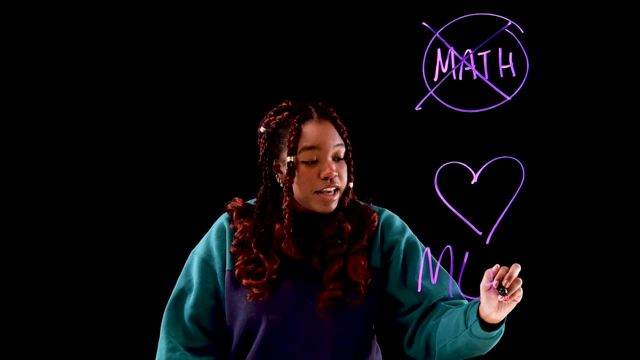 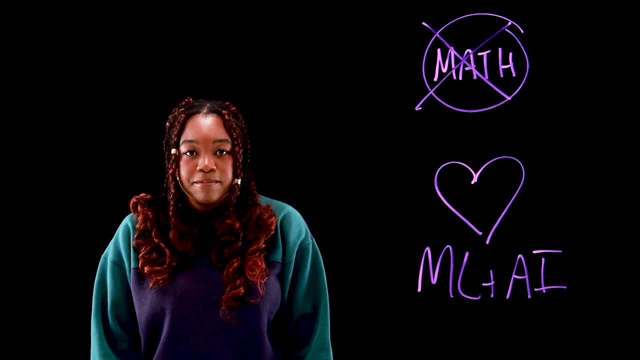 we're studying topics like machine learning and artificial intelligence. it's important for us to be able to explain to the computer how to apply mathematical concepts to large amounts of data. So one important topic in machine learning is linear regression. You may have heard of the 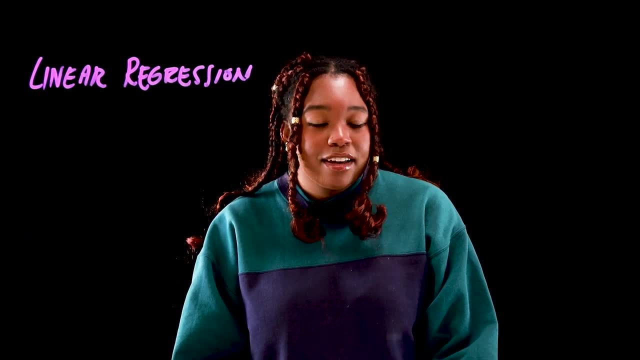 term, linear regression- and you're not sure if it's a good fit for your data set. Well, look no further. I'm going to explain what linear regression is at a basic level and give you a short summary of what linear regression is. 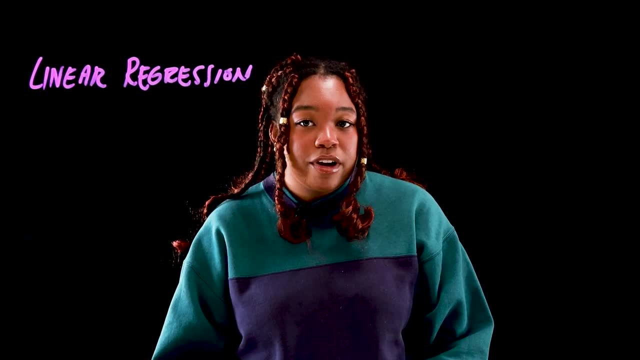 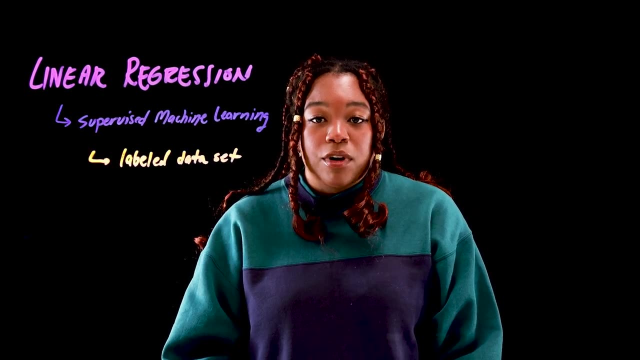 example of how it can be used in a data set with two variables. Linear regression is a form of supervised machine learning, which means that it uses a labeled data set. We're using linear regression to make predictions on continuous data, which is numerical data that can have 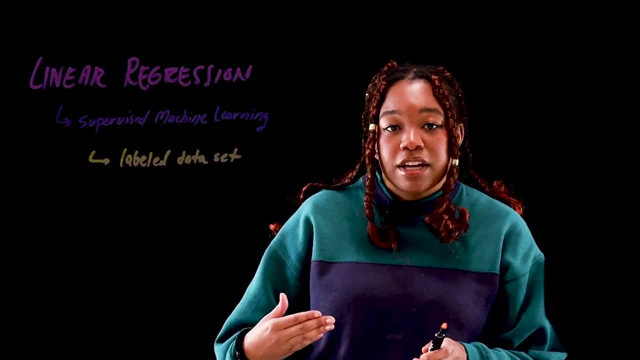 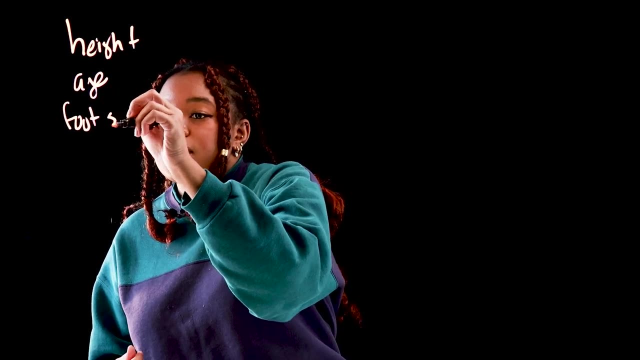 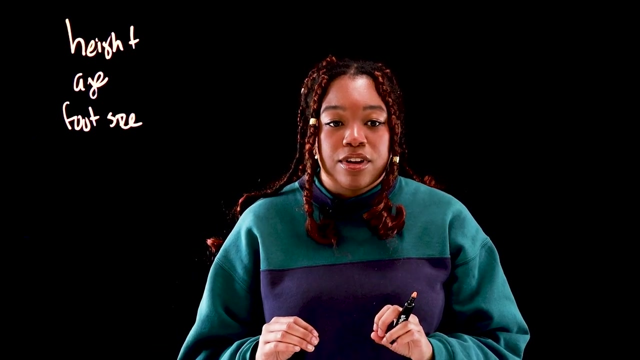 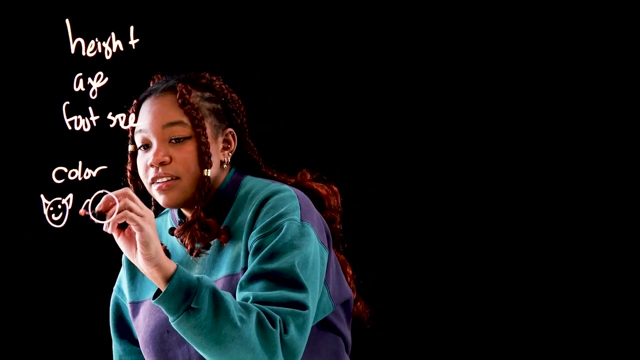 infinite values, So continuous data can be something like height or age or even foot size. This is in contrast with categorical data, which have finite distinct values. This can be things like color or the species of an animal, like a cat or a dog. These types of data would probably not be a good candidate. 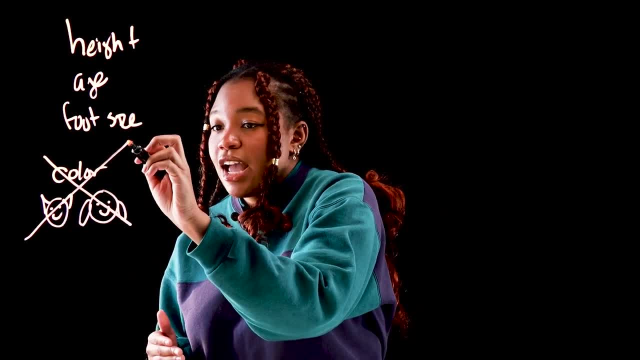 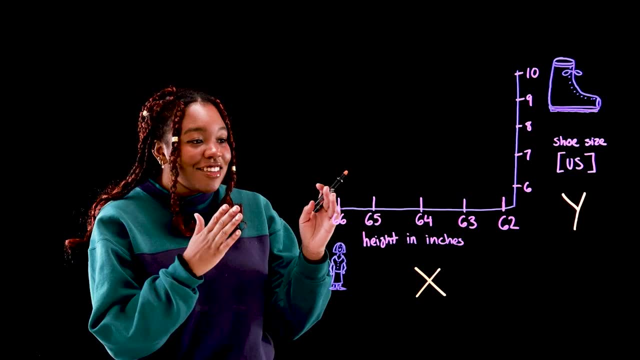 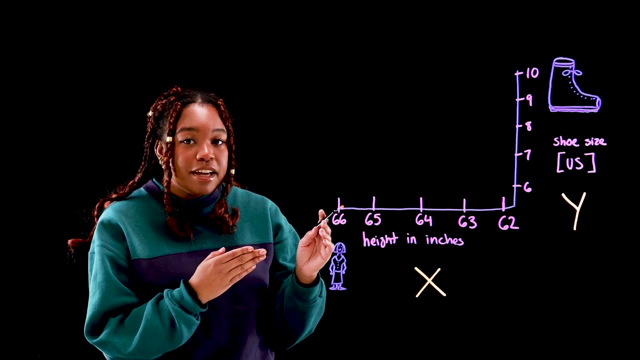 for linear regression because there are finite types of categories that they can be in. However, if your data looks like this, let's keep going. Let's take a look at this graph. Let's say, for example, we want to build a machine learning model that will identify if there's a positive